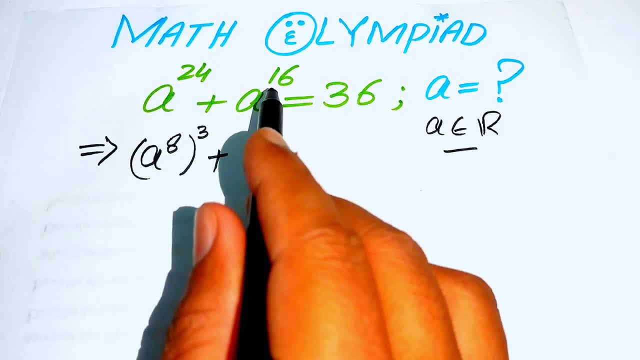 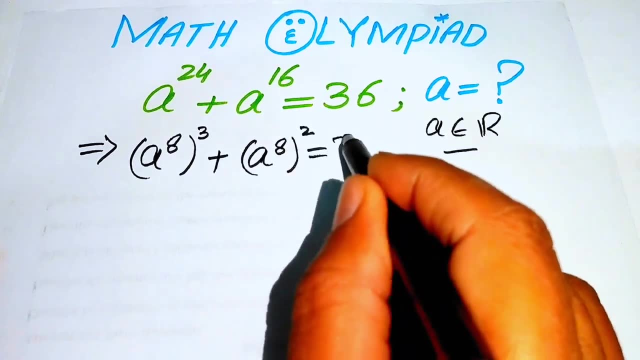 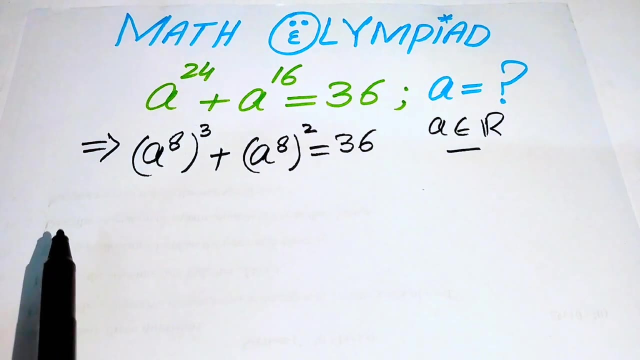 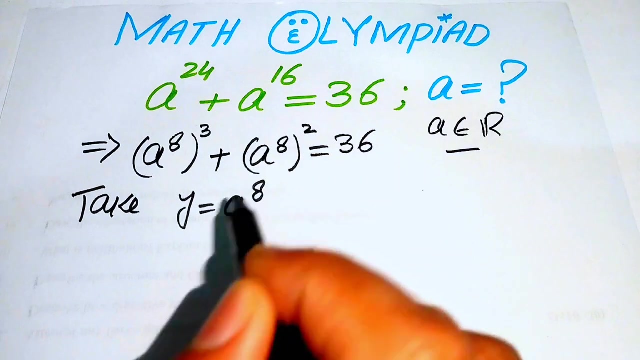 and it's whole cubed. plus we write this: a to the power of 16 as eight to the power of eight, and it's the whole square and this whole equation becomes 36.. So you see that we have a to the power of eight be the common term, so that we will take here y equals to a to the power of eight. 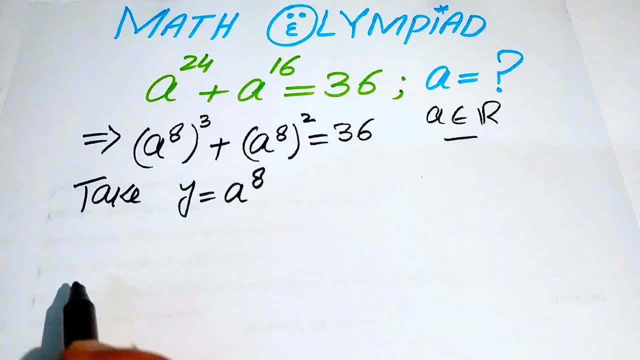 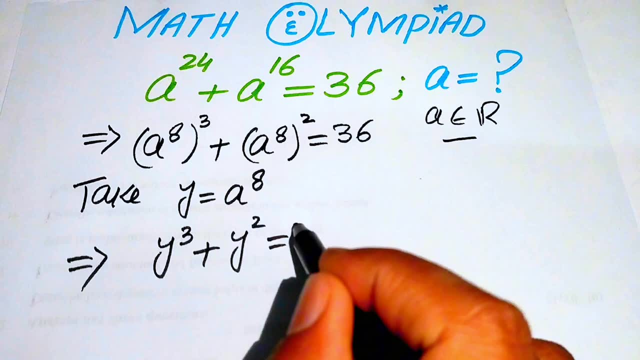 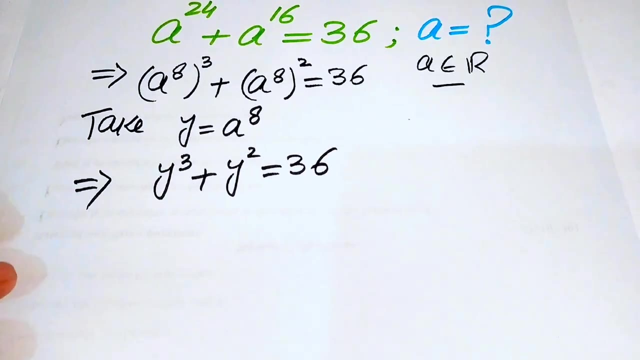 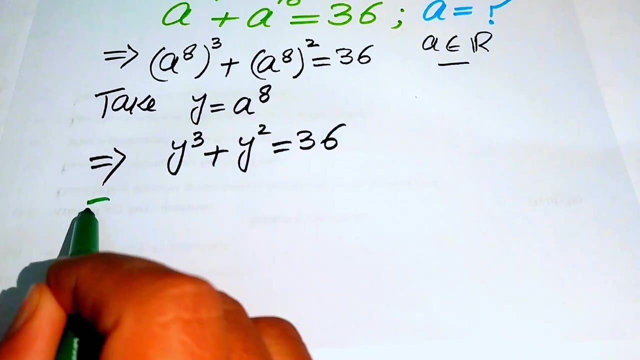 when you substitute y equals a to the power of eight in the above equation, so the above equation will becomes y cubed plus y squared equals to 36.. so in the next step here we obtain a cubic equation. so now we can make the factors of this cubic equation. so here we first rearrange. 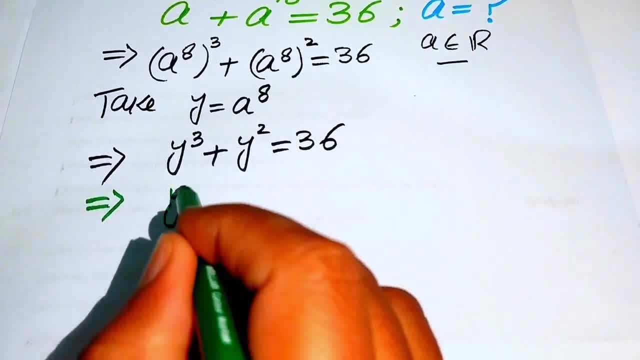 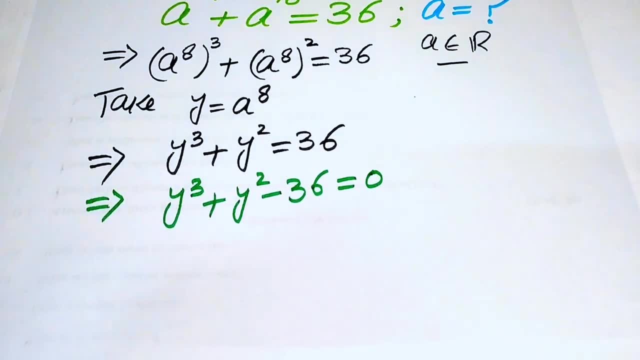 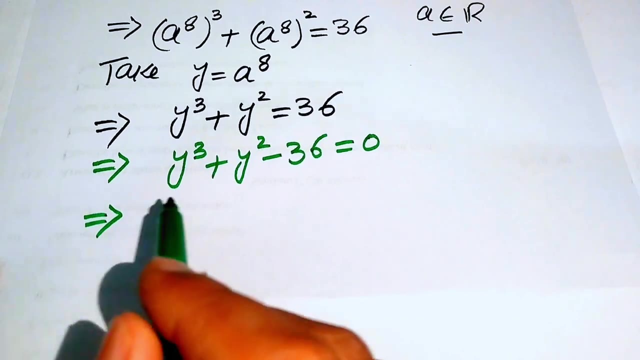 the terms and we move 36 in the left hand side and we write it as: y cubed plus y squared minus 36 equals to 0.. so now we break its middle term and we easily get the factors of this cubic equation, so that here: 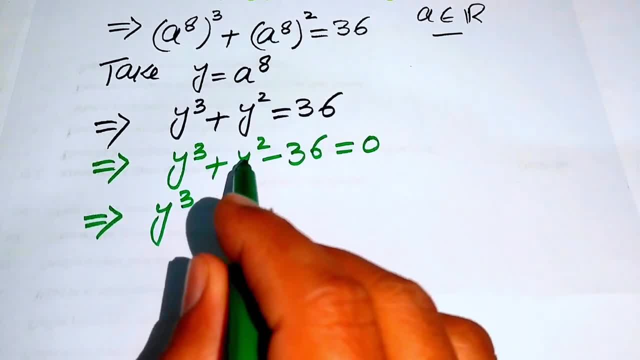 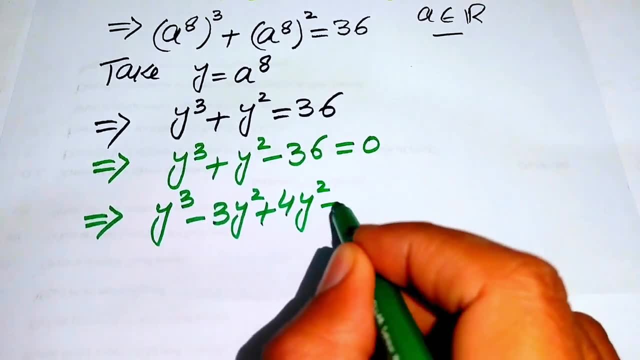 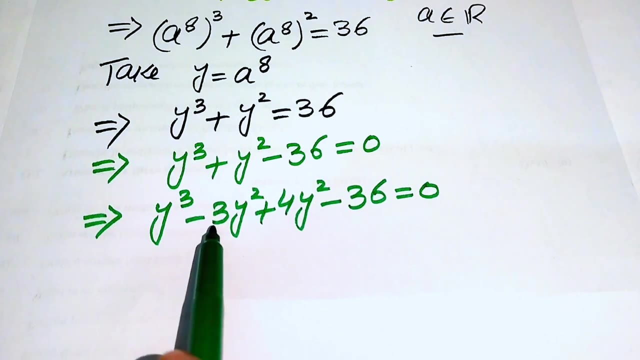 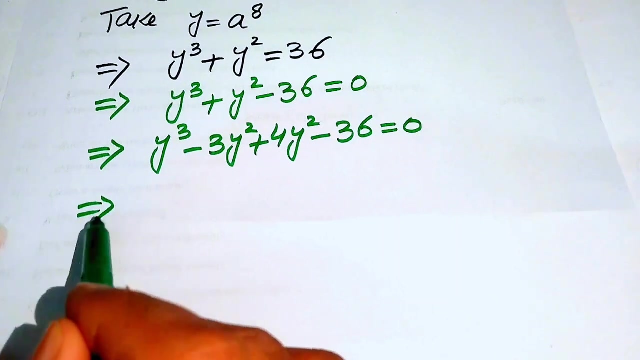 we write this y square, as we write this y square, as minus three times of y squared, plus four times of y square, minus 36 equals to 0. so because here we have plus y squared and we write it as minus 3 y squared plus 4 y squared, so it will becomes plus y square. so now we take 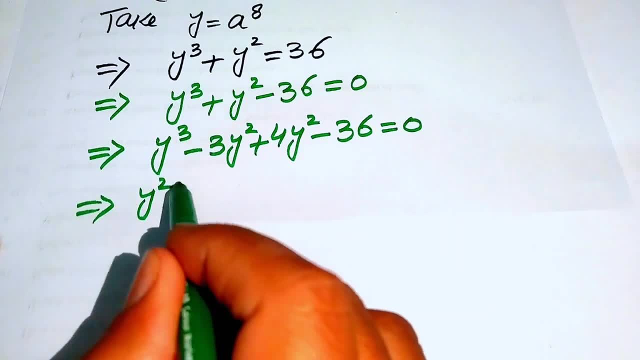 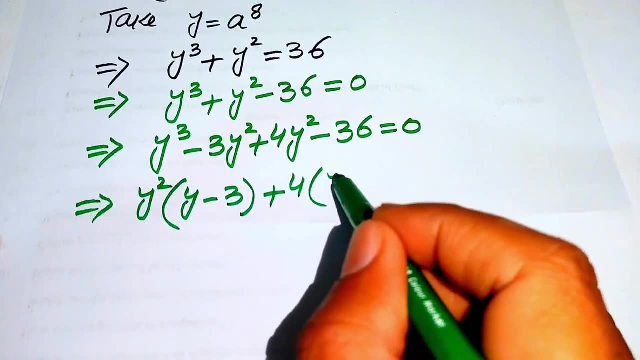 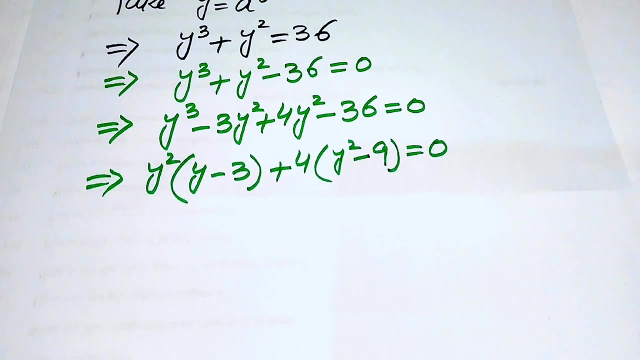 common y square from the first two terms and it will be written as square times of y minus 3. and here we take common 4 and you get y squared minus 9 and this whole equals to 0. so here we use the nice square identity and 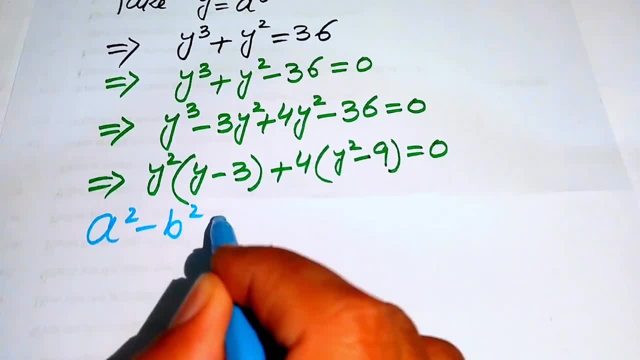 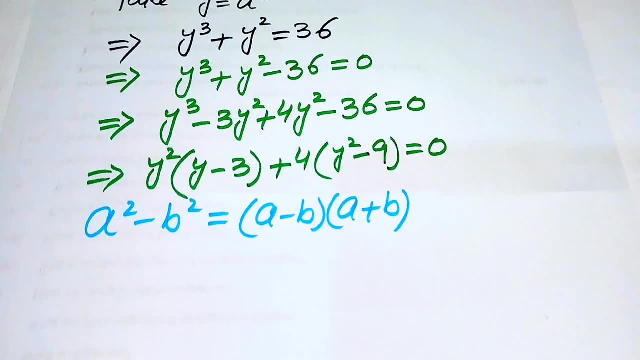 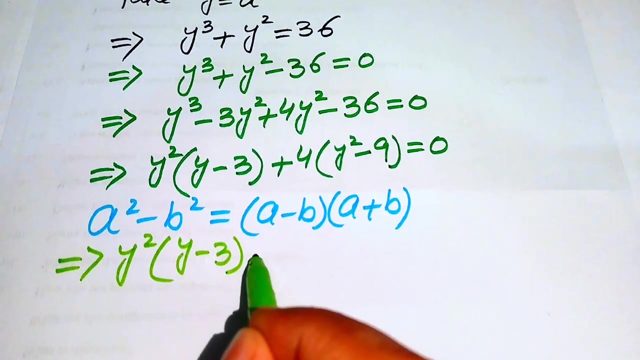 you know that if we have a square minus b squared it is equals to a minus b times of a plus b. so we use this square identity in the above term and our above equation will becomes in this form: y square into y minus 3 plus four. 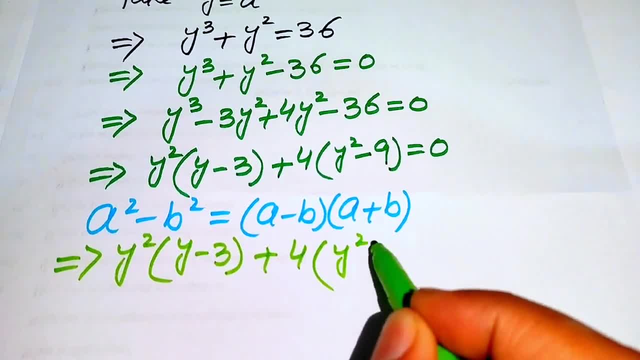 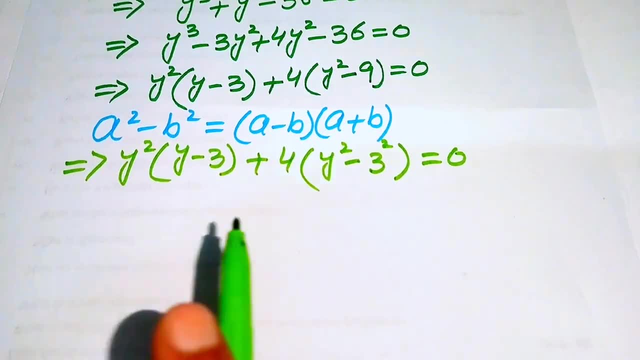 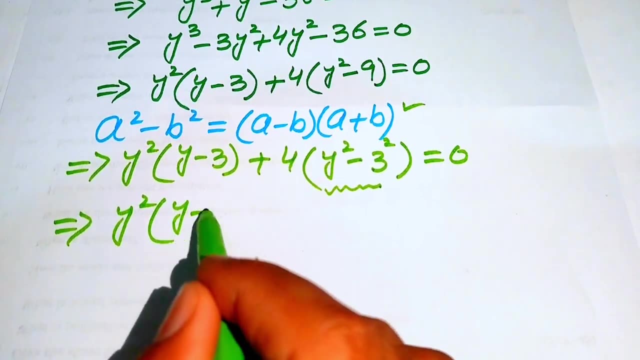 times of first, we write this equation as y square minus, we write this 9 as 3 square and this whole equation equals to 0.. So here we use this nice identity on this term and we write it as y squared into y minus, 3 plus 4 times of. 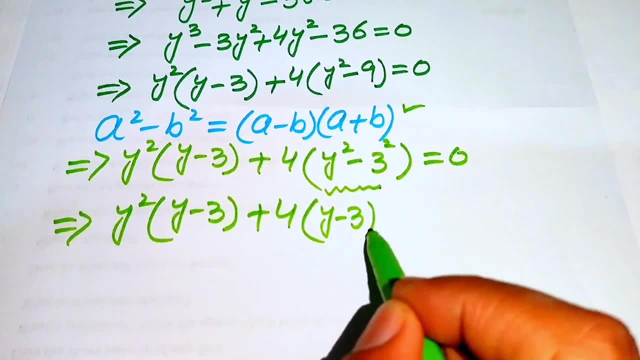 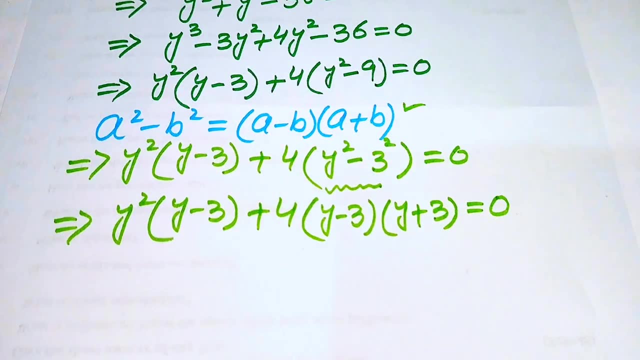 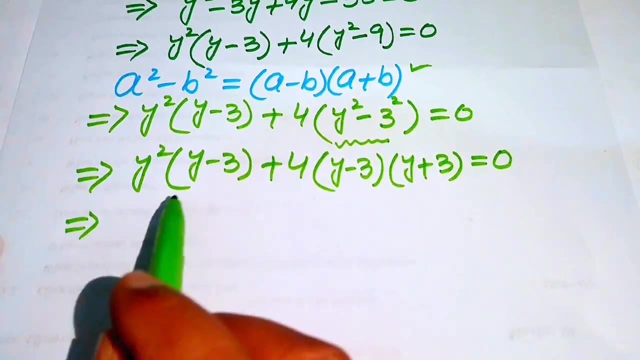 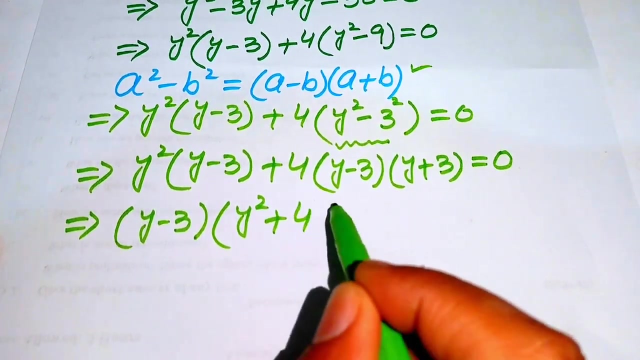 y square minus 3 square becomes y minus 3 times of y plus 3. so here we use this nice identity and this whole equals to 0.. so here you see that we have y minus 3 be the common term from both of these terms and we write it as y minus 3 times of y square plus 4 times of. here we take common y. 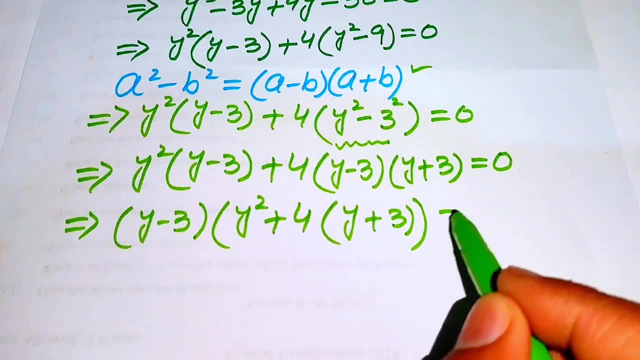 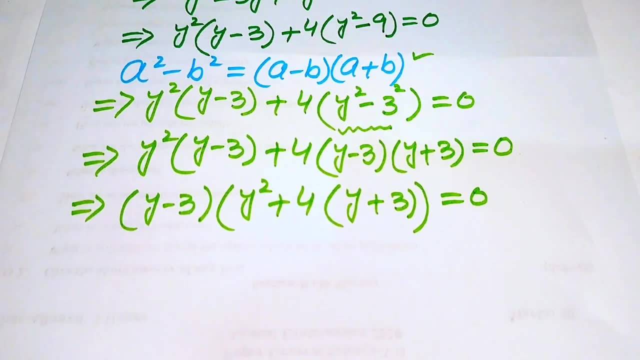 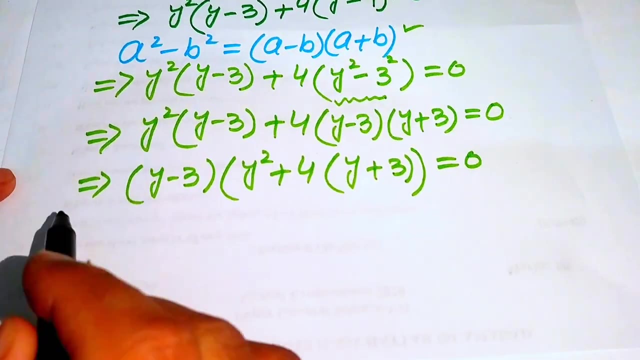 minus 3 and we get y plus 3 and this whole equation equals to 0. so that in the next step we convert this equation into the two cases. so our first case is we write: y minus3 equals to 0 and our under planets equation equals to 0. in the third case we write that we convert this equation into the two cases. so our first case is we write: y minus 3 equals to 0. 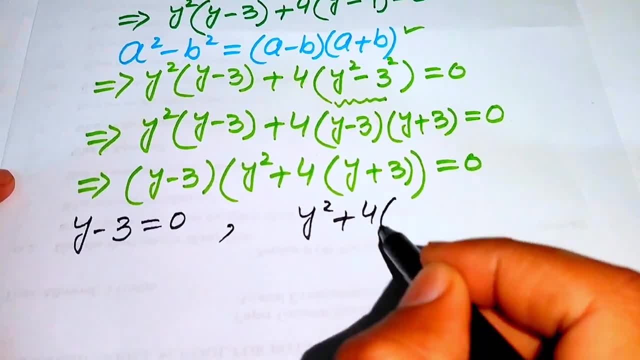 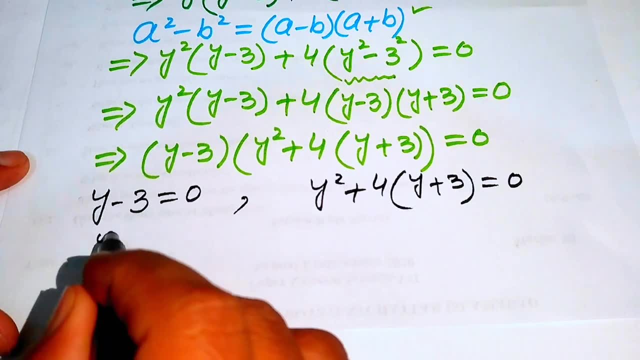 and the second case is we write y squared plus 4 times of y plus 3 equals to 0. so in the first case we easily get the value of y. so here we move this minus 3 to the right hand side and we get y. 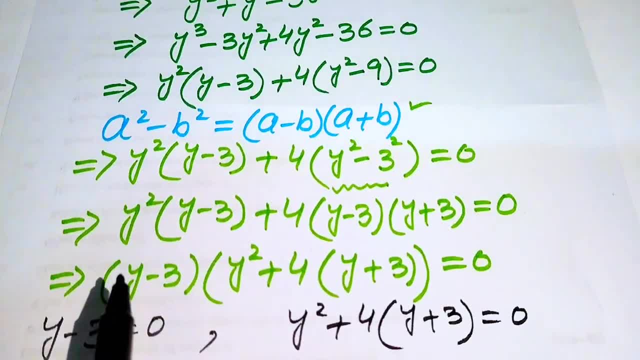 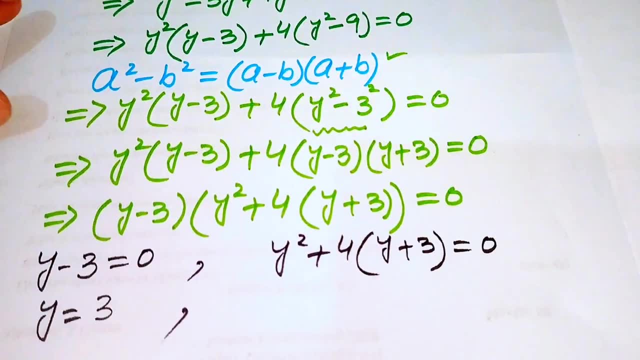 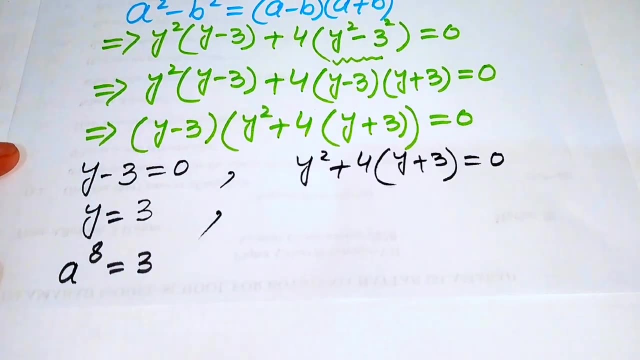 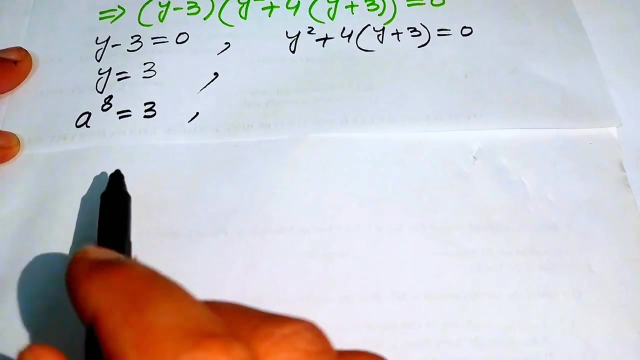 equals to 3. and here we back substitute the value of y and you see that we will take our y equals to a to the power of 8. so we substitute this value of y here and you get a to the power of 8 equals to 3. so in the next step, so here we get a to the power of 8, equals to 3. but our target is: 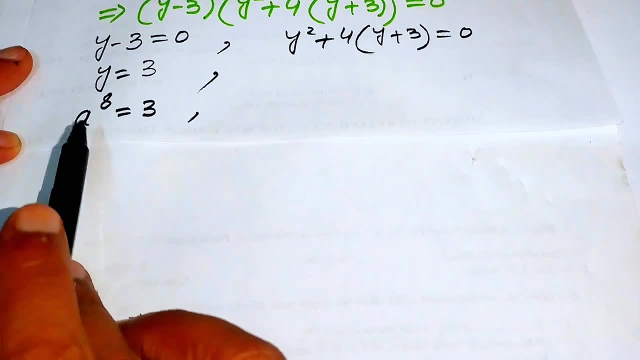 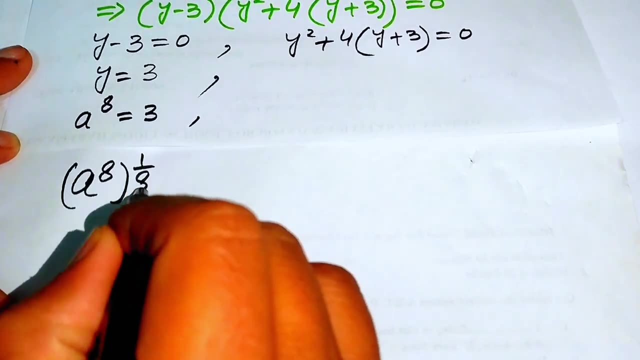 to find the value of a. so here we take the eighth root on both of the sides and we write it as a to the power of 8, and it's so sofort. so we can take our left hand side as a to the power of 5 and we put our total解 with 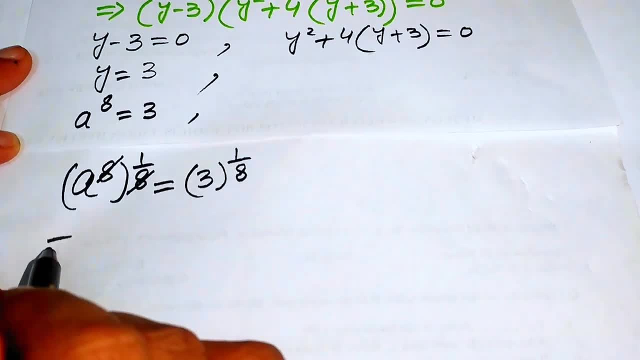 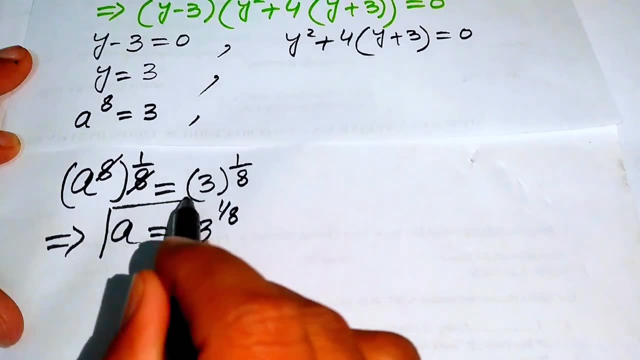 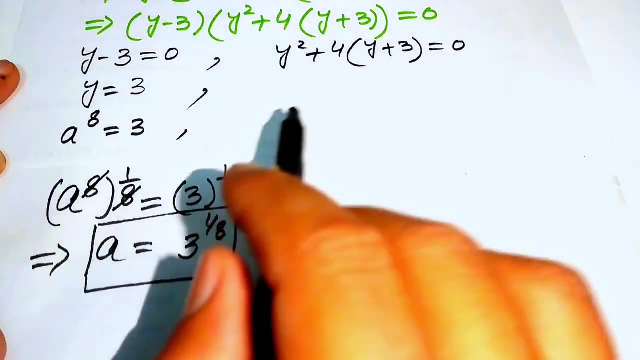 the whole power, 1 over 8 equals to 3 to the power of 1 over 8. so here you see that this 8 are cancelled out by this 8 and we get a equals to 3 to the power of 1 over 8. so this is the value of b. 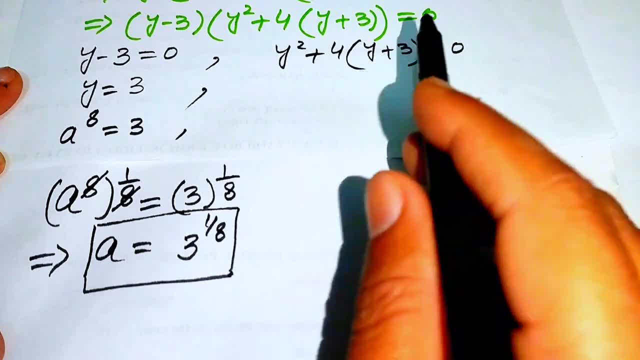 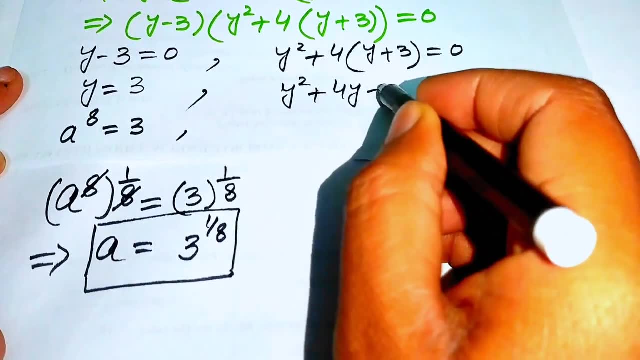 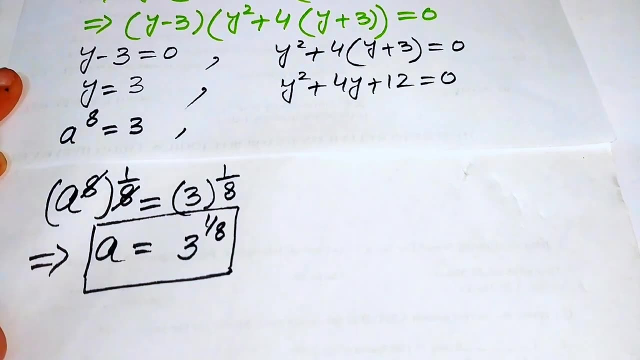 so now, in order to find the other values ofa, we need to solve this quadraticった now. first we, and we multiply this 4 on both of these terms and we write it as y squared plus 4 times of y plus 12 equals to 0.. so here we need to find the real roots. so first we check: is this quadratic? 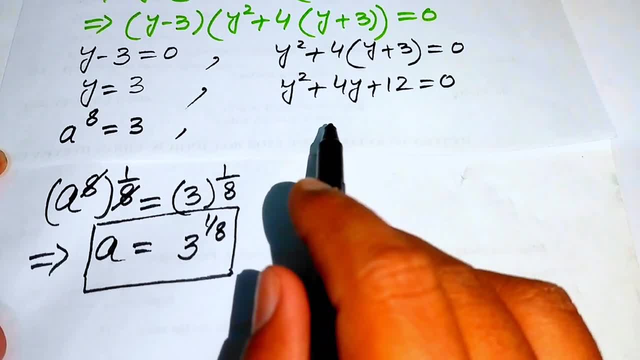 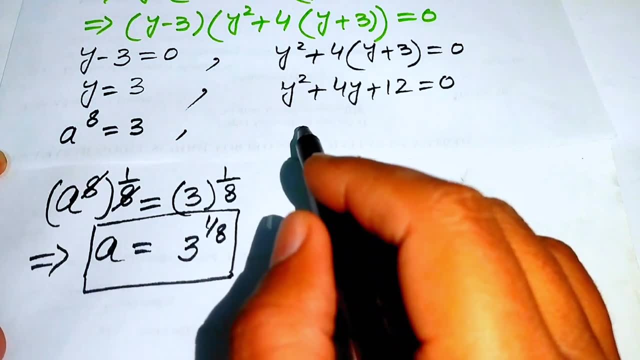 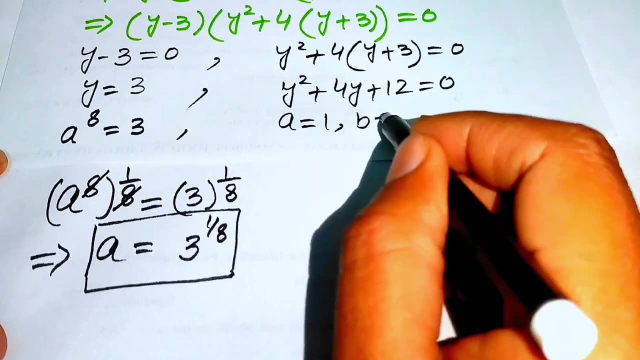 queen has real roots or not? by using the quadratic formula or, sorry, by using the discriminant formula. so you know that in order to use the discriminant formula, first, we need the coefficients of this equation, and these are: a equals to 1, b equals to 4 and c equals to 12 and discriminant. 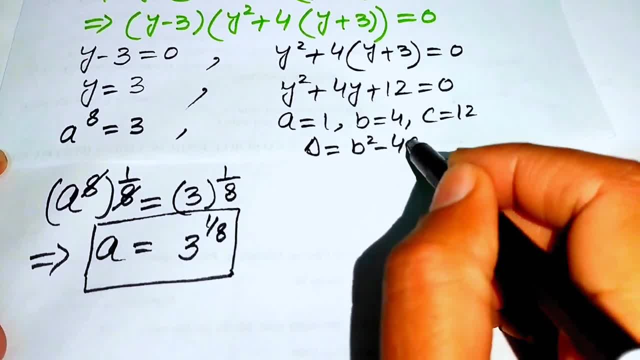 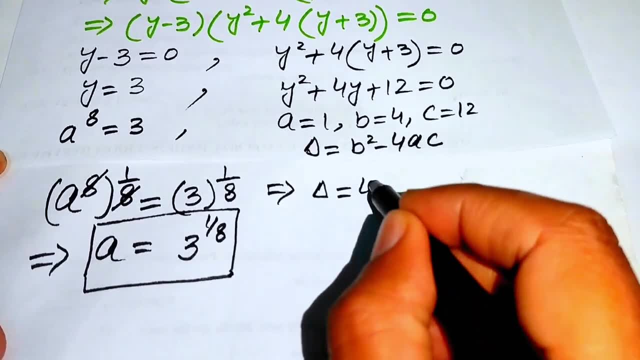 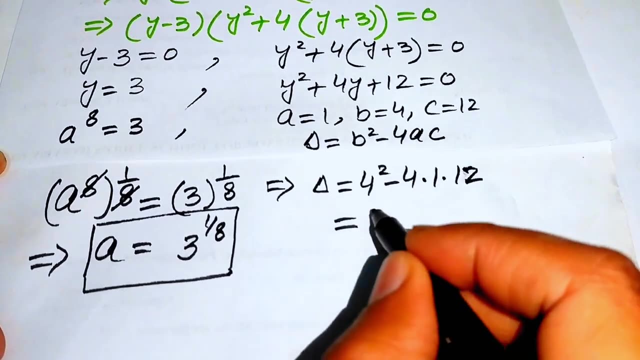 formula is written as: delta equals to b squared minus 4 times of ac. so here this delta will becomes: the value of b is 4 square minus 4 times of a is 1 and c is 12.. so 4 square is 16 minus. 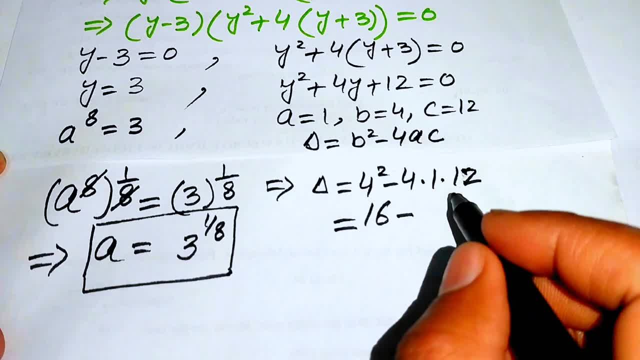 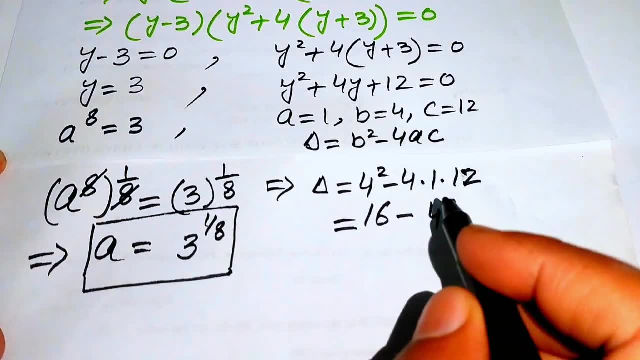 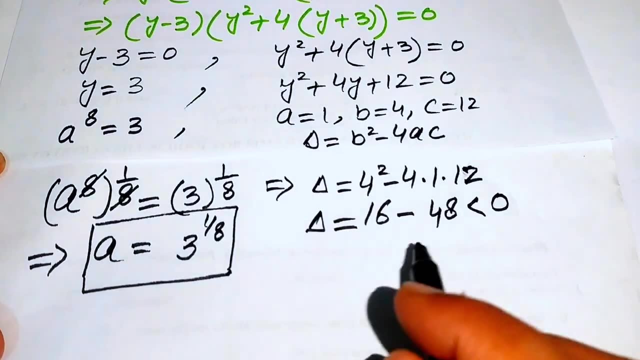 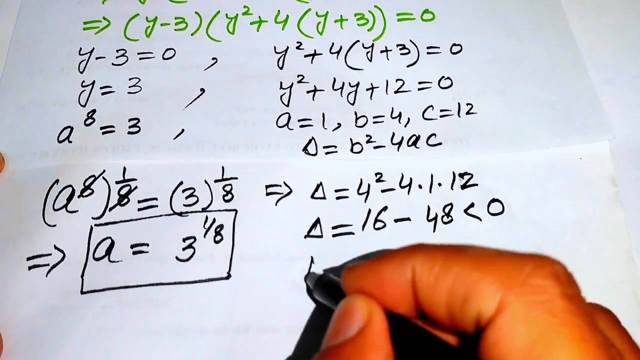 4 times of 12 is equals to 48. so when you subtract 16 minus 48, then you easily see that it is lesser than 0.. so we know that if our data is less than 0, it means that this quadratic equation has no real 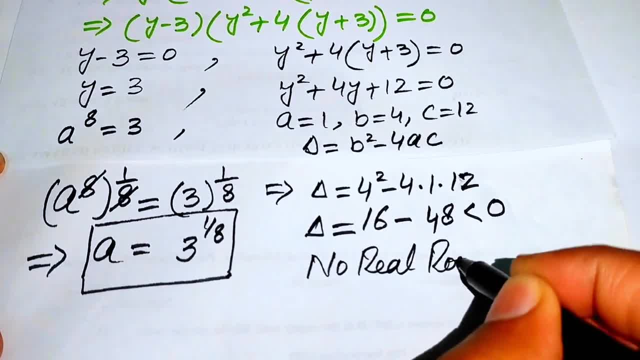 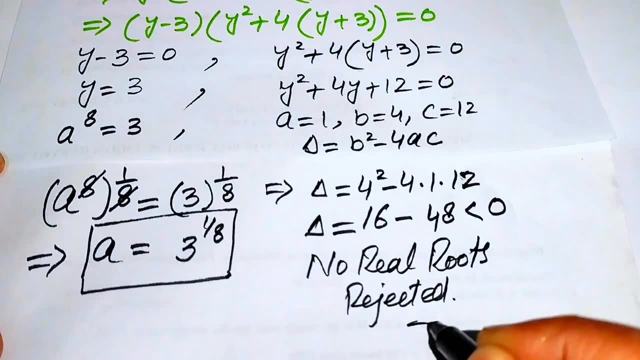 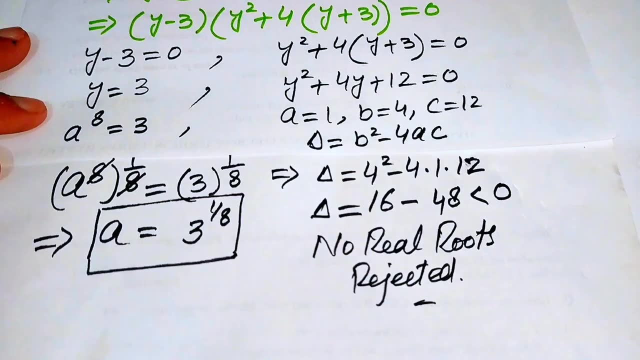 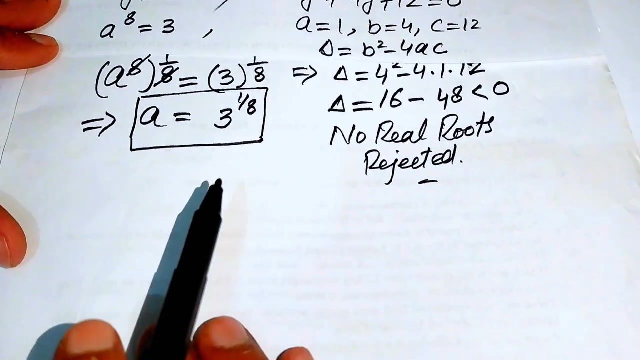 root. so if data queen has no real root, so that we will reject it this case, because in this question we need only real solution- so so that here we we have just only one solution of this equation, and this is a equals to three, to the power of eight. so in the next step we will just check this solution.